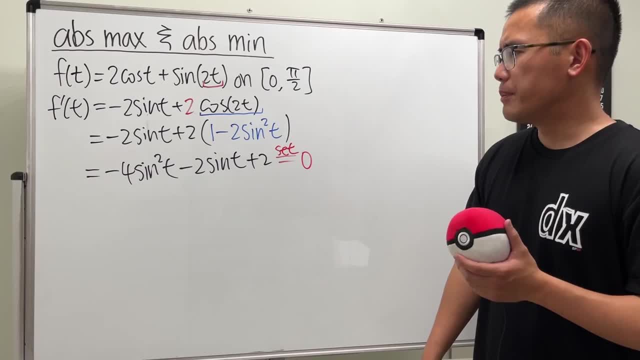 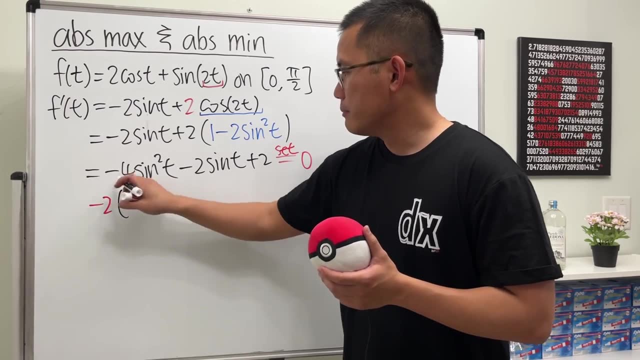 And it's a quadratic. We are going to factor it And perhaps let's factor out negative 2 first for everybody. It's easier that way. So let's see: Factor out negative 2. And we get positive 2t sine t. 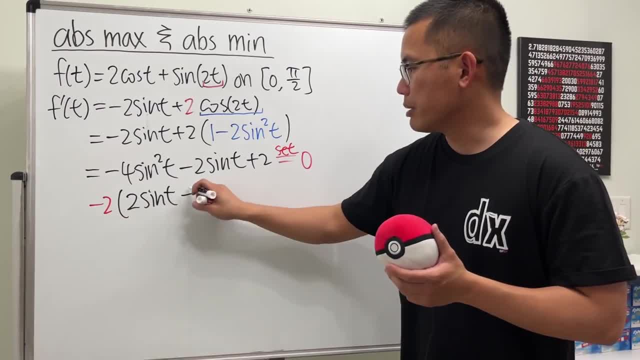 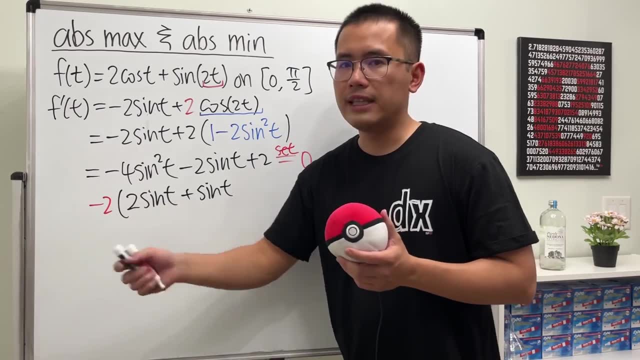 We have the negative 2 here, but we took it out already, So it would be a plus. And then this is sine t, And then this is positive 2.. Factor out the negative 2.. It's like dividing by negative 2.. 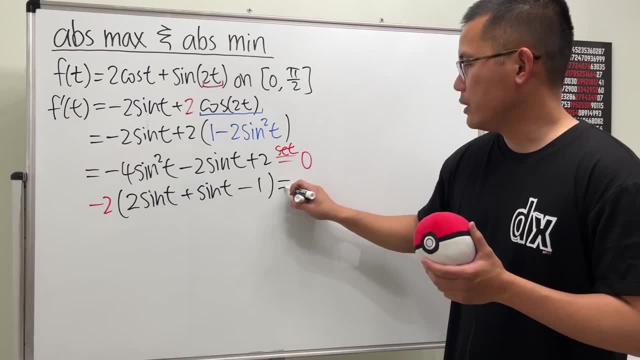 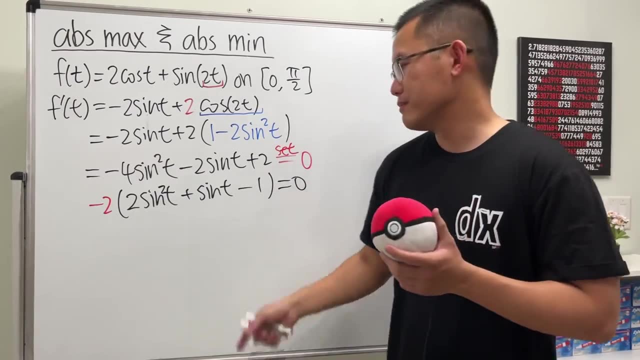 So we have minus 1.. All right, And that will be equal to 0.. Now we can do this. By the way, this is sine squared. We can do this by factoring, Because it is a quadratic And it works. 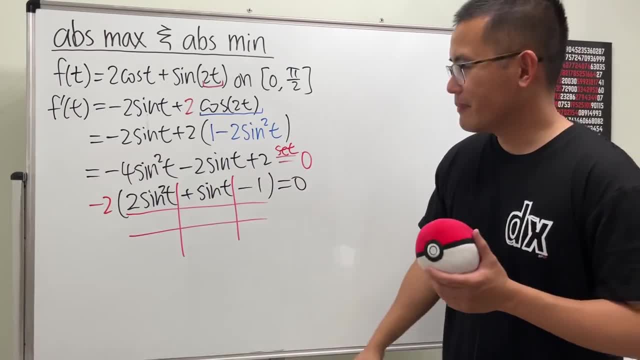 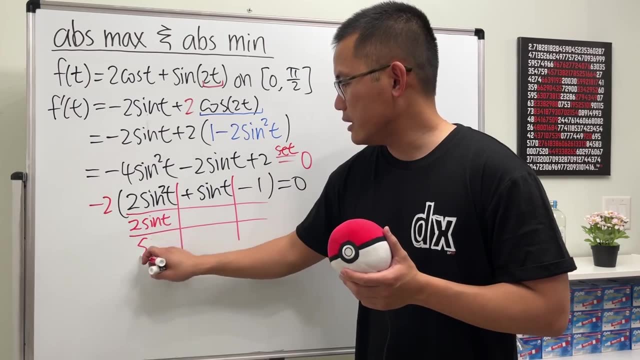 I'll show you guys my favorite tic-tac-toe method. Okay, What times 4 gives us 2 sine squared t? Well, we need 2 sine t times sine t. That works wonders. And then we have to think about what times 4 gives us negative 1.. 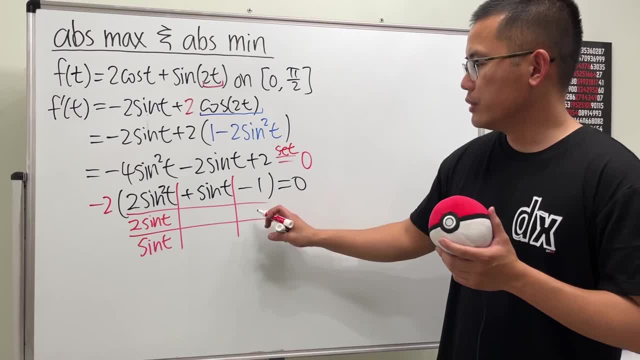 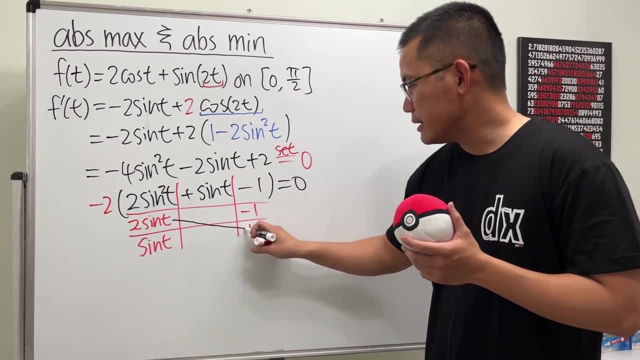 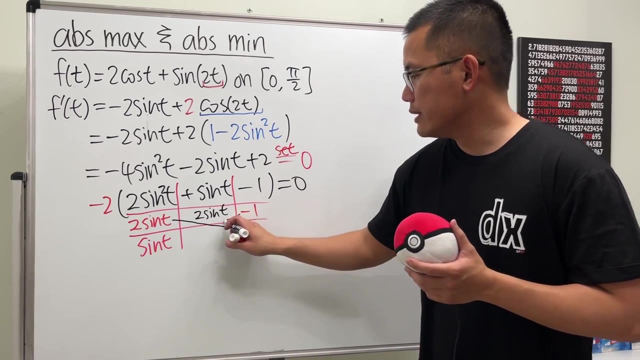 And the order matters. We are going to put 1 and negative 1, with the 1 thing right here and negative 1 right here, Because this times this is how we check And it will give us 2 sine t And then, when we do this times that it gives us negative sine t. 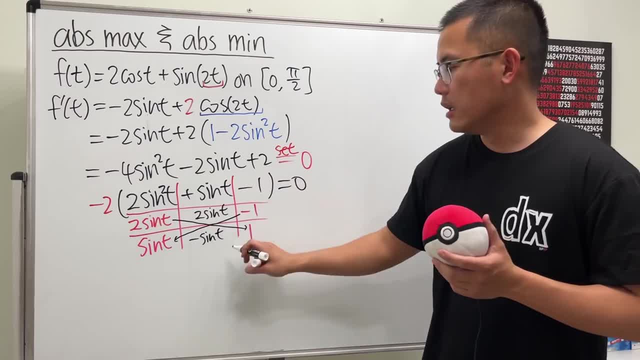 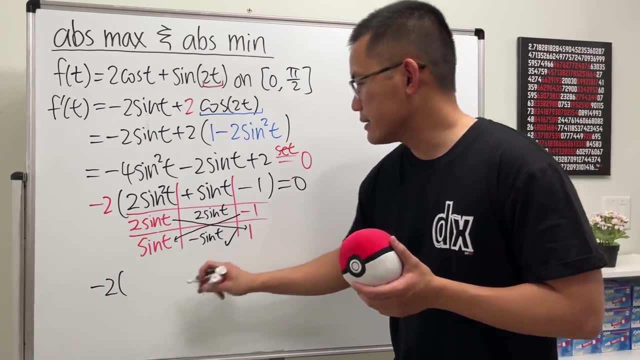 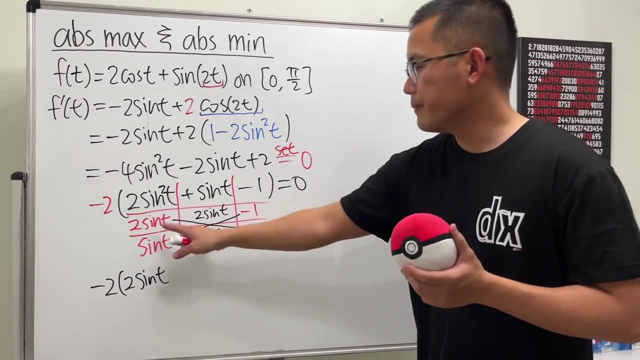 Together we get positive sine t And we got the correct combination. So altogether we get negative 2 times this minus that, So 2 sine t. And when you use this, when you write down the answer, you go across. 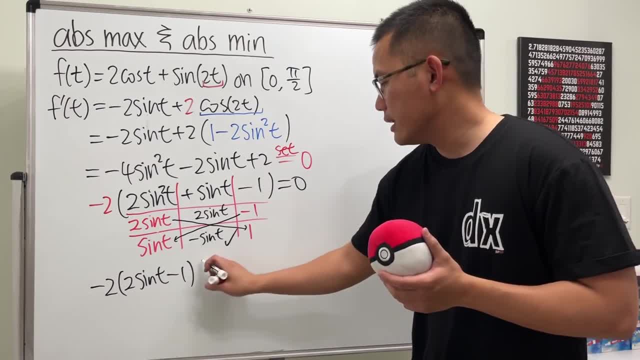 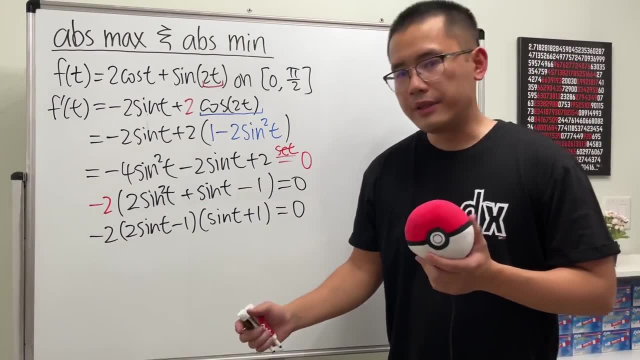 So 2 sine t minus 1, and then sine t plus 1.. And we make this equal to 0.. All right To continue. we have to make this factor equal to 0. So we can put a minus 1 to the other side. 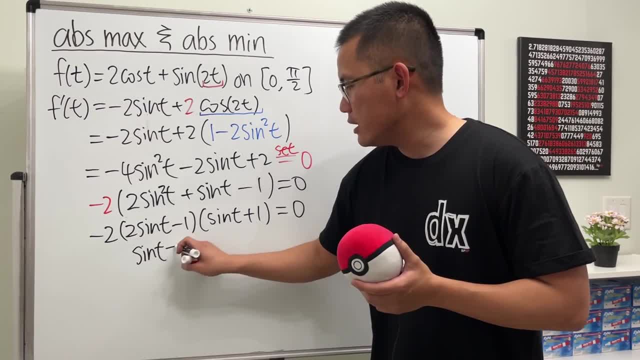 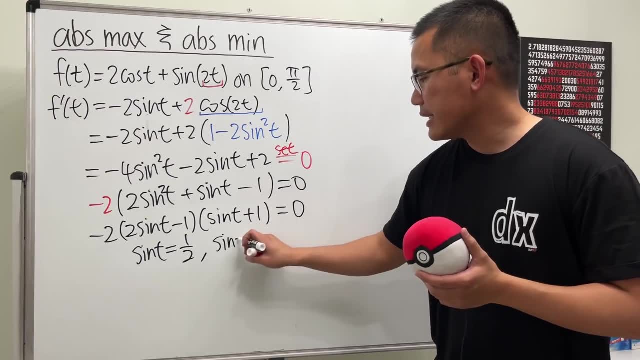 And then divide the 2 on both sides, So we get sine t being equal to 1 half, And then put this to be 0. We put the 1 to the other side, So we get sine t being equal to negative 1.. 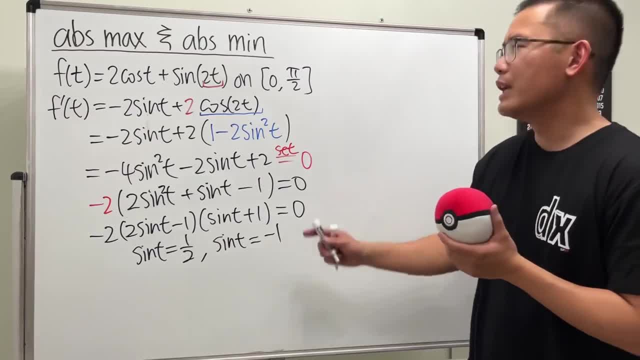 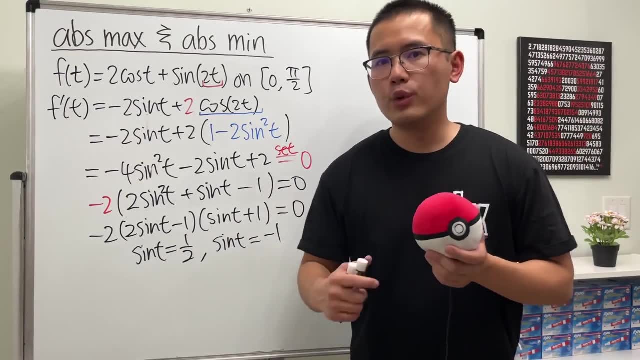 And now we just have to solve these two equations, And the good news is that we just have to solve them on this interval. Have a look: Sine t being equal to 1 half, We can use the reference triangle method And I will remind you guys that, on the side, 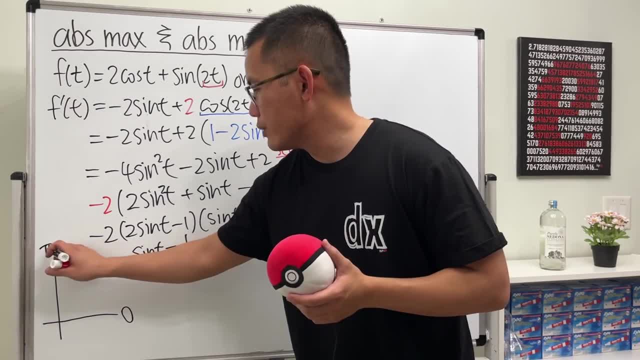 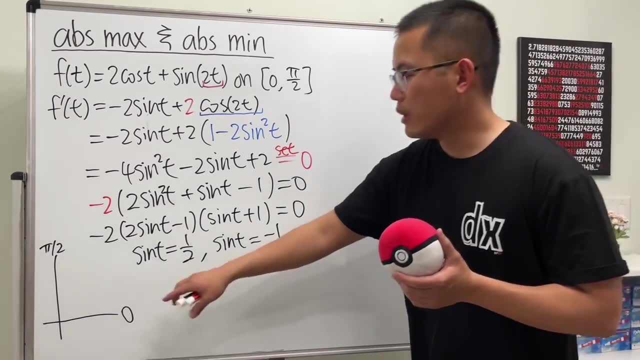 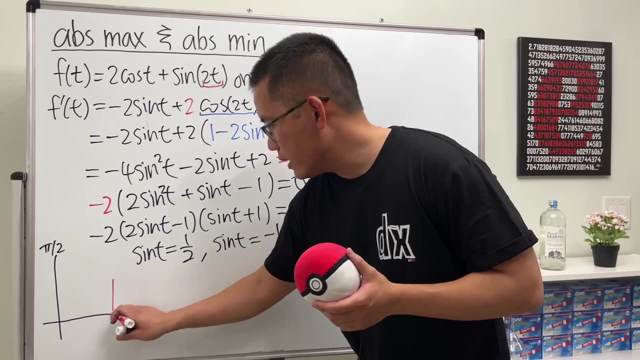 OK, So here is 0 radius And here is pi over 2 radians, namely 90 degrees. Sine is opposite over hypotenuse, Or on the xy plane. it is the same as saying y over r, So we can take 1 to be the y. 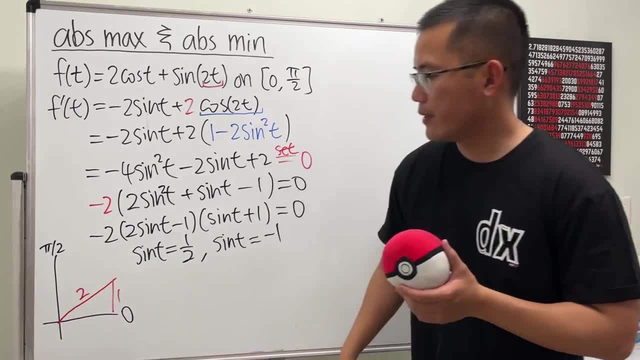 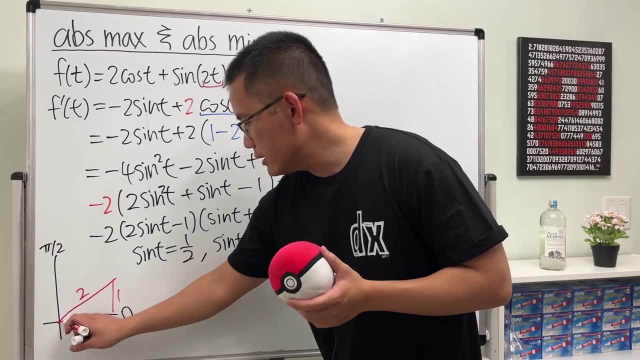 And then r is just 2.. All right, So we have a right triangle And this is, in fact, a 30-60-90 special right triangle. This is going to give us square root of 3.. And the most important thing is that you have to know this is the shortest side. 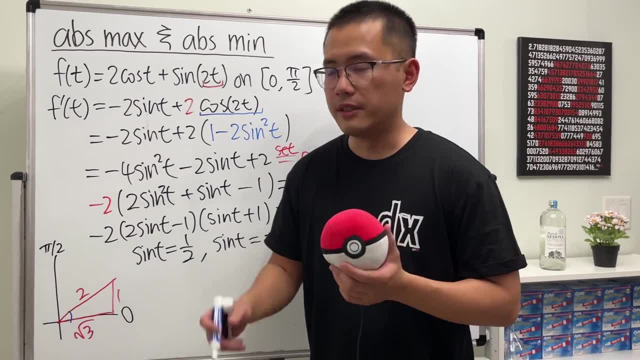 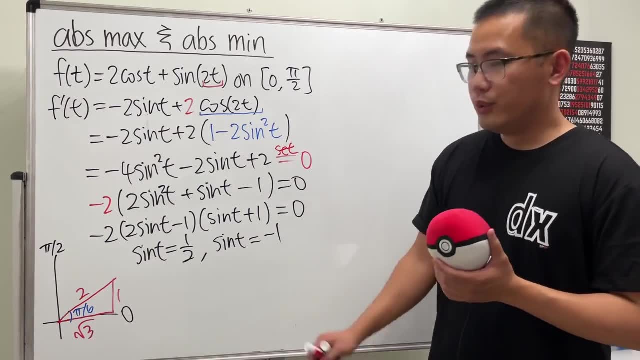 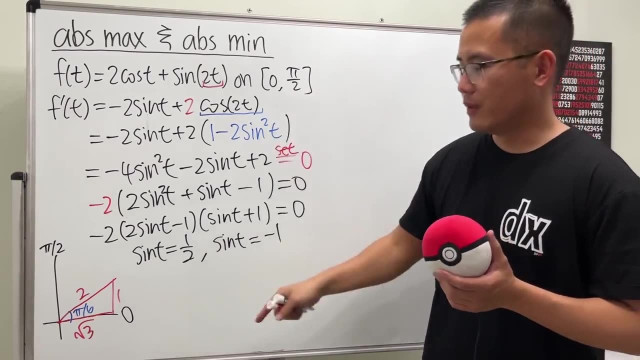 So this is the smallest angle, which is the 30 degrees, And 30 degrees is pi over 6. And that's all we need Usually this right here. we will have to get infinitely many solutions, But no, We just need the solution on this interval, which is that 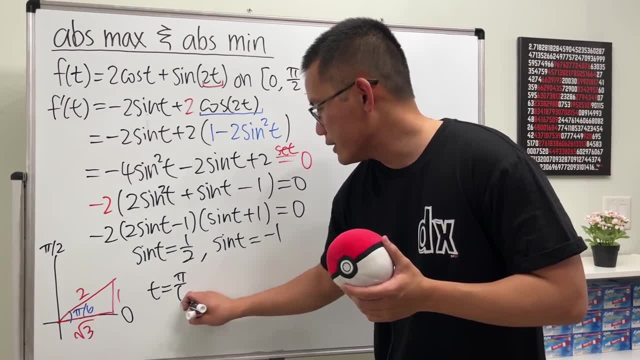 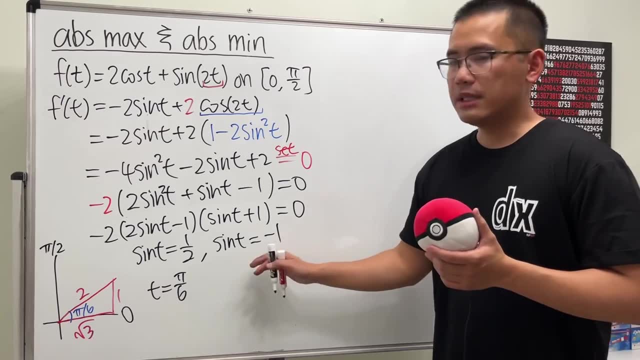 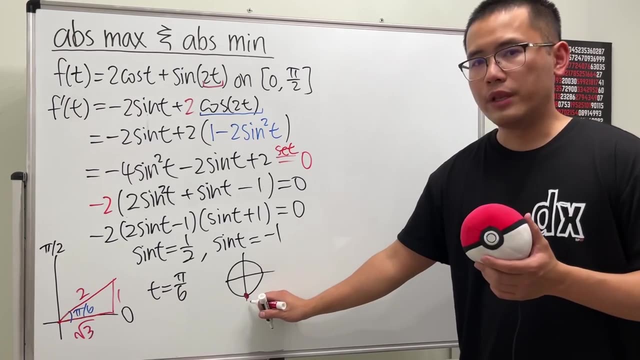 So t equals pi over 6.. And for this one sine t is equal to negative 1.. Well, sine is the y-value on the unit circle. You can look at it here. This is where the negative 1 is for the y-value, which is the sine value. 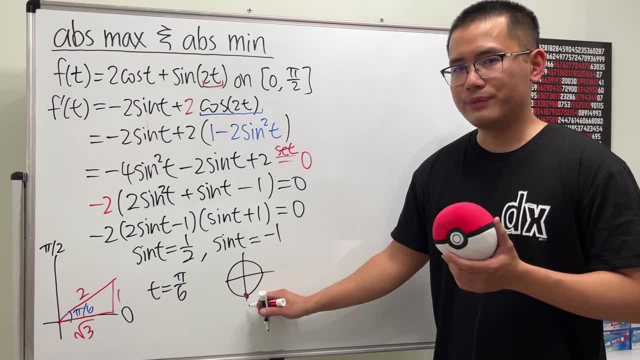 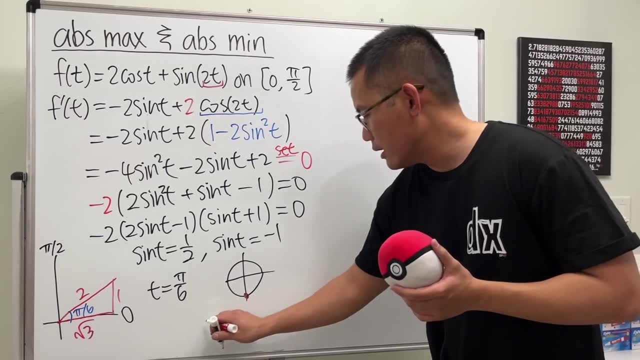 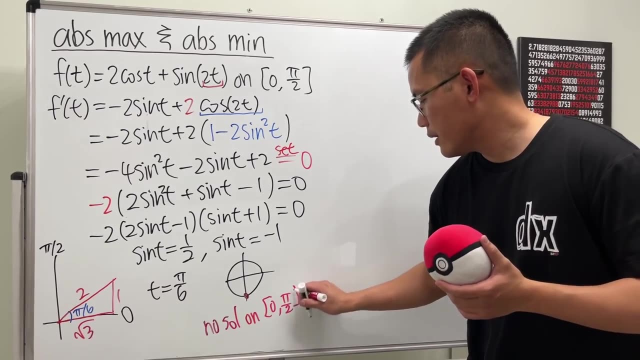 But this is 3 pi over 2, or negative pi over 2.. So we don't have to consider that. So I will tell you no solution on the interval 0 to pi over 2.. So this is our only critical number, cn. 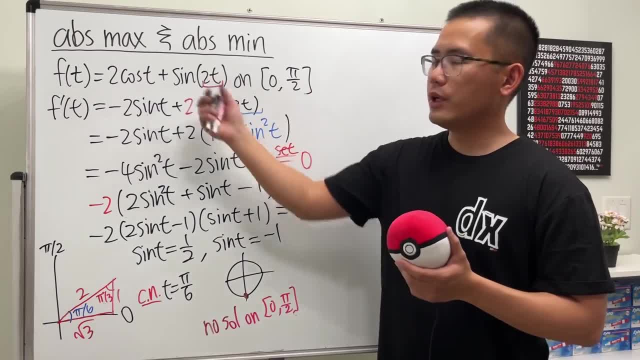 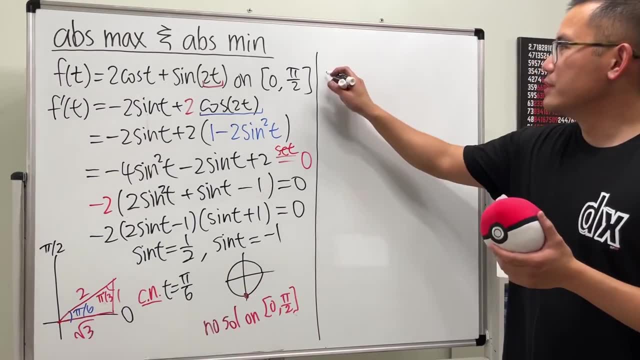 OK, right now we just have to plug in this, this and that back to the original function and see which one is the biggest and which one is the smallest. So here we go. Let's do the critical number first. So we have f of pi over 6.. 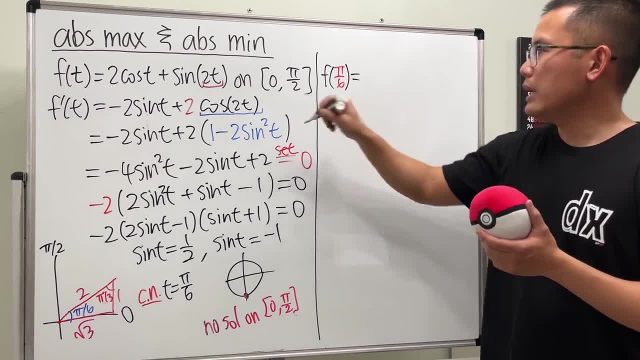 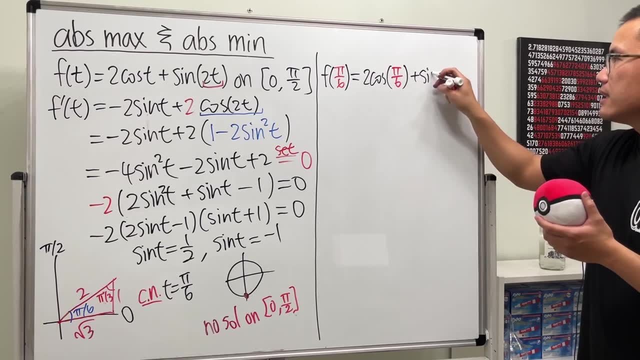 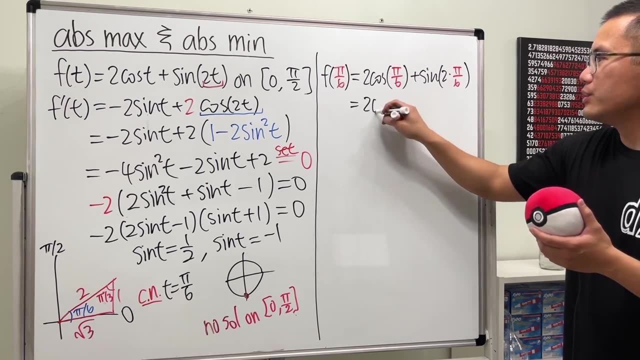 And this will give us 2 times cosine of pi over 6.. And then we add cn, So we have sine of 2 times pi over 6.. OK, this is just 2 times cosine of pi over 6. And this is sine. 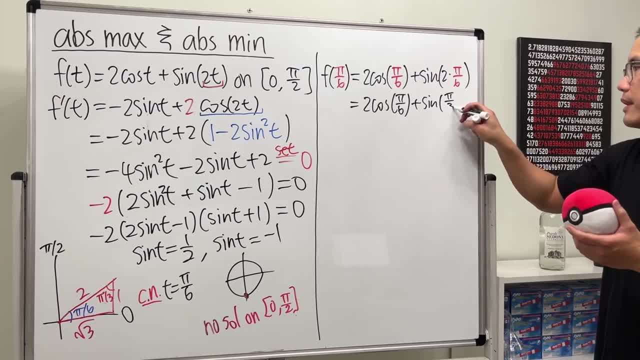 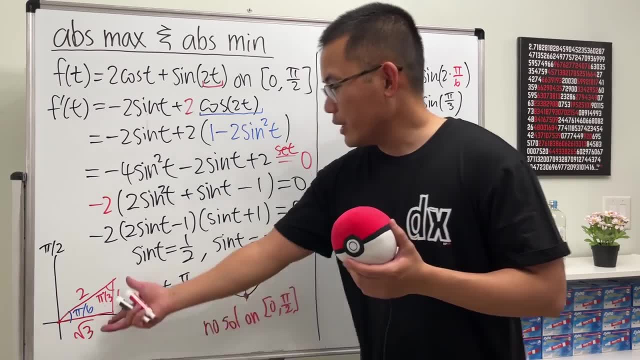 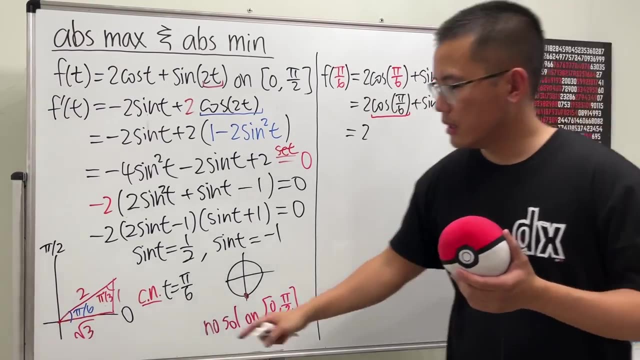 And then we can reduce this and that which is pi over 3.. And you can see that this angle is actually pi over 3 because that's 60 degrees. So we can use that triangle to help us out with this. First we have 2, and then cosine of pi over 6.. 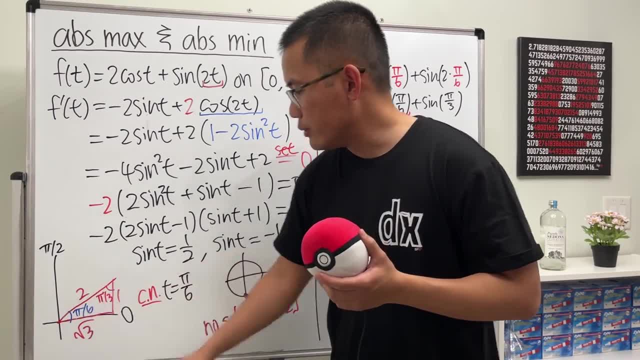 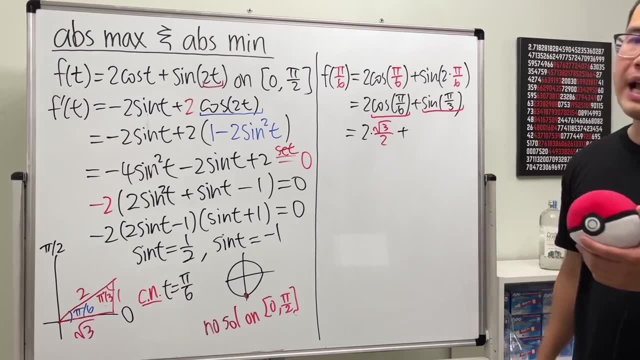 Look at this as the angle and do adjacent over hypotenuse. So we have square root of 3 over 2. And then next we add sine of pi over 3. We look at this angle and do opposite over hypotenuse. 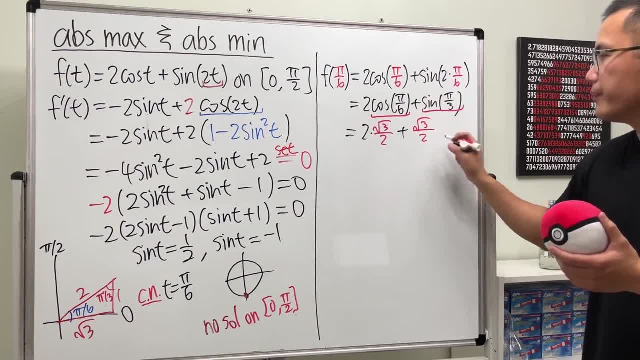 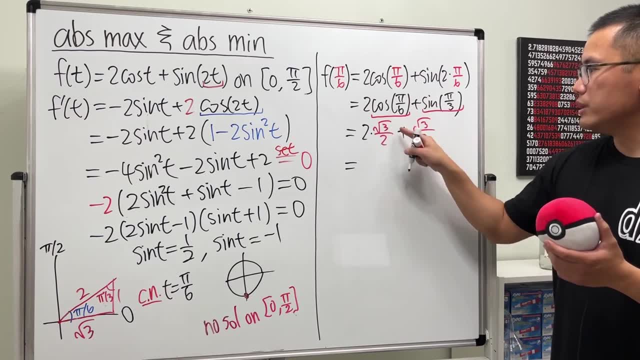 So that's also square root of 3 over 2.. And they have the same denominator so we can just add the top together. So in fact, 2 square root of 3 plus 1 square root of 3, we get 3 square root of 3.. 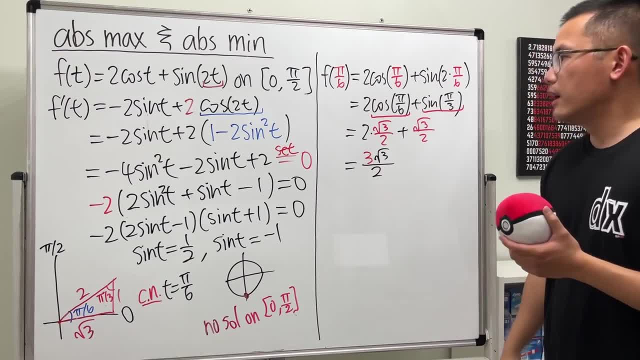 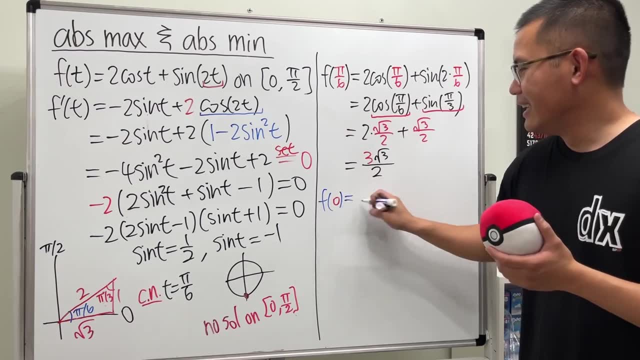 And then over the same denominator, which is 2.. OK, and then continue. Let's go ahead and check 0, which is the nicest number. Put 0 into the original, so we have 2 times cosine of 0.. 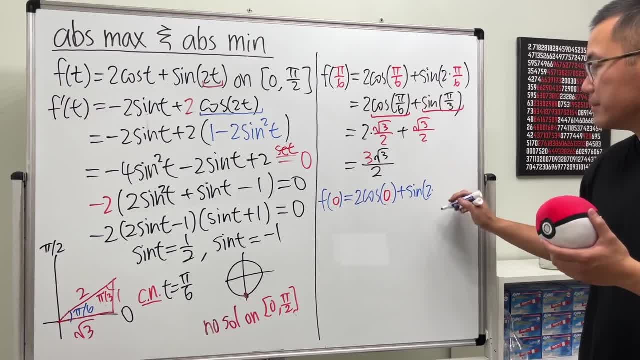 And then we add sine of 2 times 0. Sine of 0 is just 0.. Cosine of 0 is 1.. 1 times 2.. All together we get 2.. And lastly, we check pi over 2.. 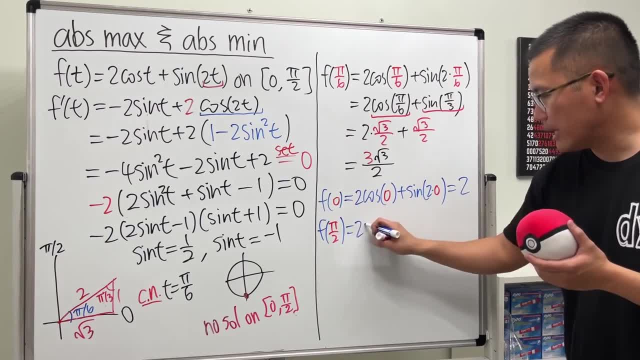 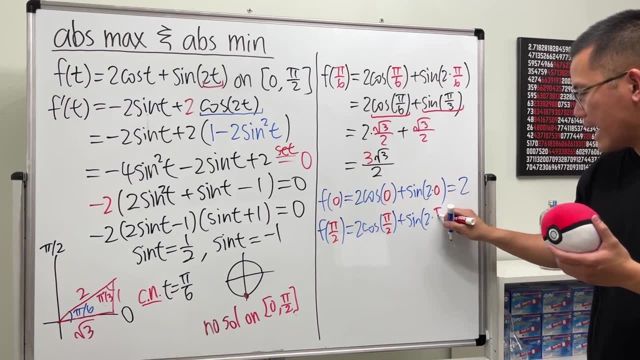 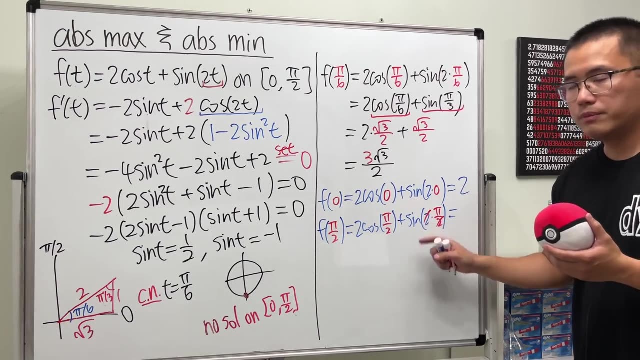 So this is 2 times cosine of pi over 2.. And then plus sine of 2 times pi over 2.. Check this out. This and that cancel Sine pi is 0.. Cosine pi over 2 is also 0.. 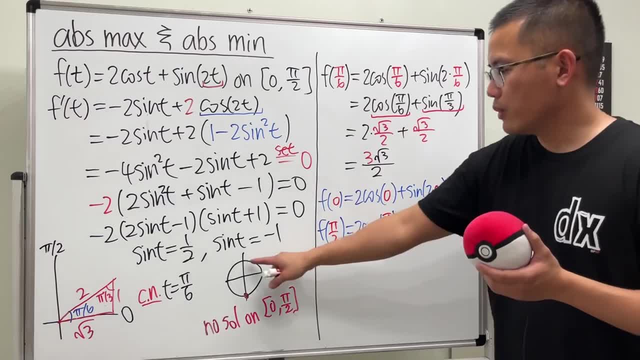 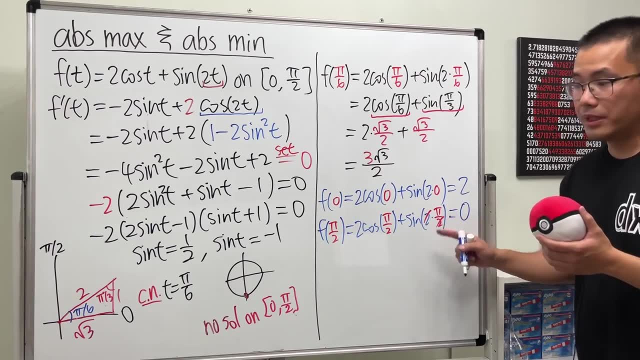 Because we look at the x value right here, which is 0.. So 0 plus 0 is just 0.. And, by the way, sine pi is 0 because we look at the y value right here, which is 0.. 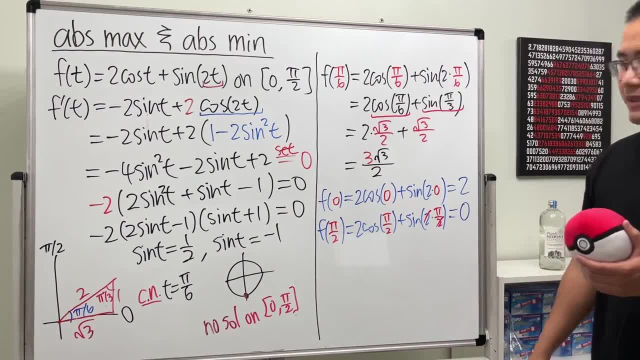 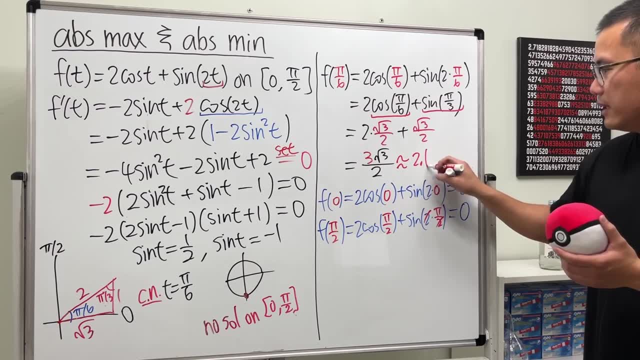 OK, we have all the things that we need. Which one is the biggest? Is it this or that? Let me tell you, this one is bigger And, if you would like, you can use the calculator and you will get approximately 2.6..